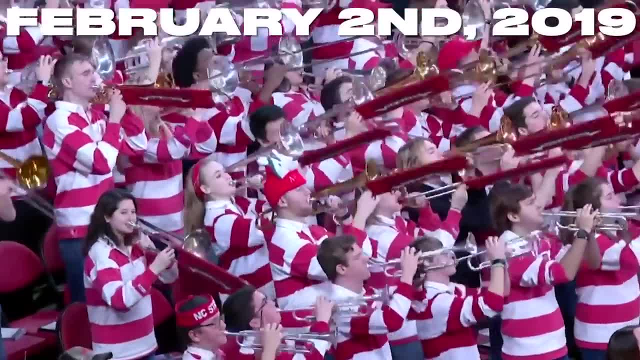 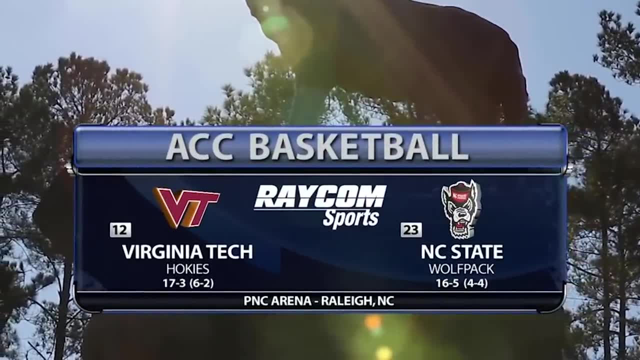 the worst college basketball game, February 2, 2019.. Rally North Carolina. The 12th-ranked Virginia Tech Hokies have traveled to North Carolina to take on the 23rd-ranked Wolf Pack. NC State comes into this game 16-5, but they're still looking for a marquee win to stay. 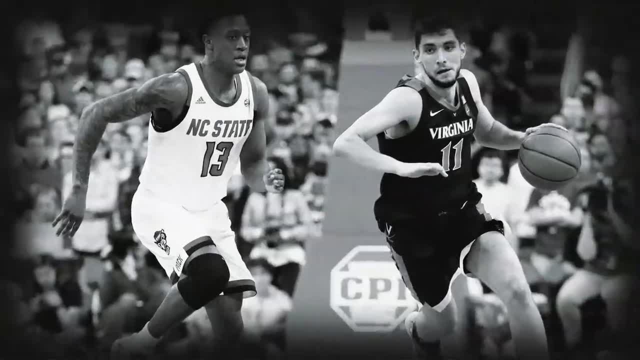 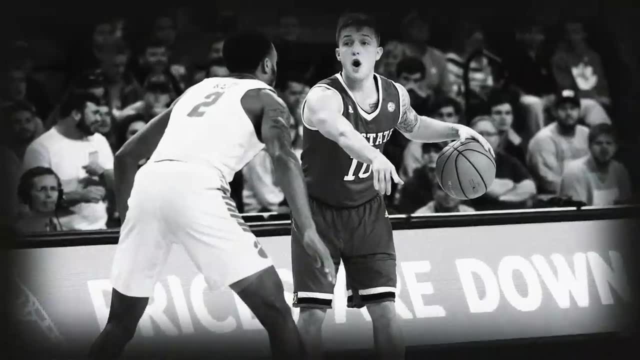 on track and prove they deserve to make it into the tournament. Just last week they took 3rd-ranked Virginia the distance, losing by just one in overtime, 3-2.. Three days before that, Wolf Pack guard Braxton Beverly dusted off Clemson with a 3-point buzzer. 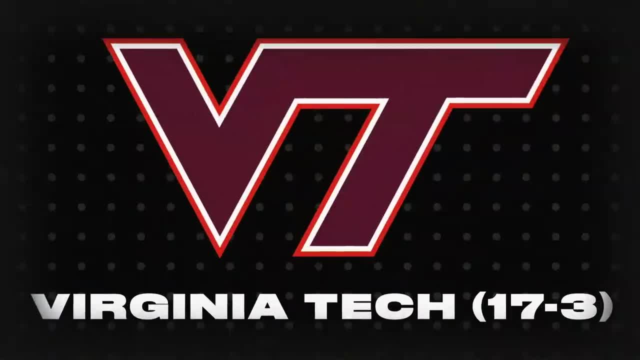 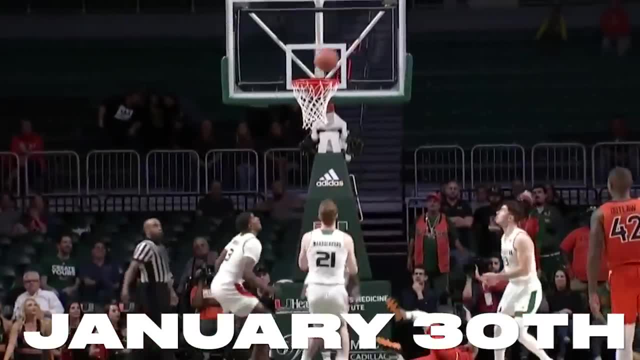 beater. They've got talent and the chance here to make a statement. Virginia Tech is 17-3, and also looking to keep up their momentum heading into February. The Hokies are good on offense, but they're coming into the game without their star guard, Justin Robinson, who suffered a toe. 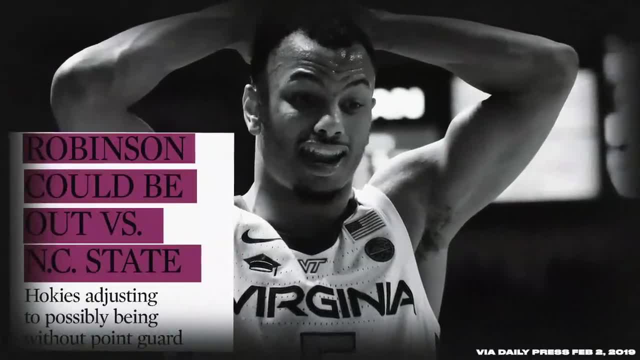 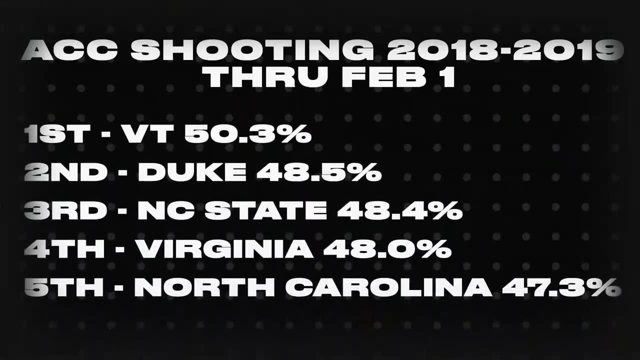 injury against Miami in the game prior and an otherwise thin bench. It'll be a challenge, but a road win here for Tech would be huge. So this is a big game for both teams who are jockeying for position in a competitive ACC. And also these teams are first and third in the ACC in shooting. 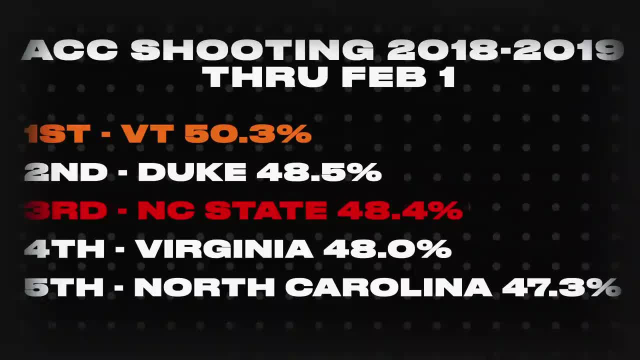 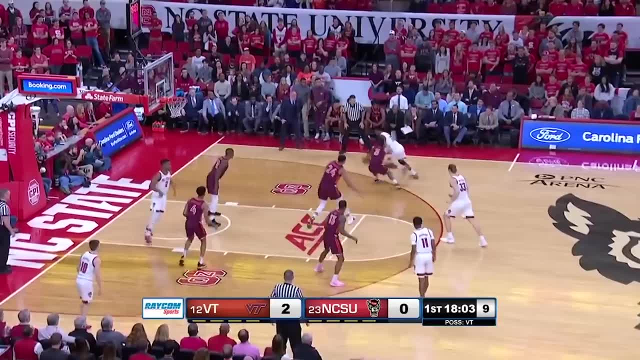 which is worth mentioning, especially in a conference dominated by powerhouse programs like Duke, UVA and UNC. The game starts and the Hokies kick things off with a jumper from Carey Blackshear, The Wolf Pack respond with one-and-kind from CJ Bryce. 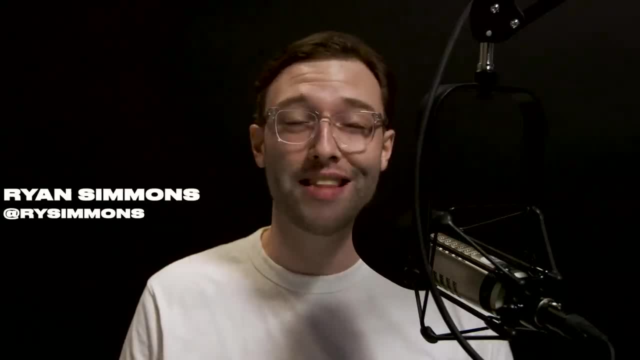 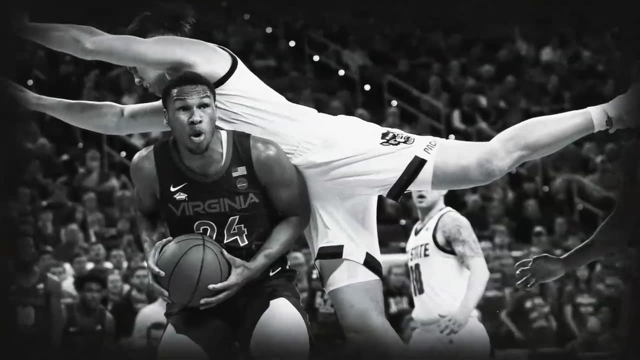 Viewer, congratulations. You just witnessed the only points that either of these teams will make in the first seven minutes of this game. Though you are about to see it with your own eyes, it's possible to account for why these teams just cannot put the ball into the hoop, Except. 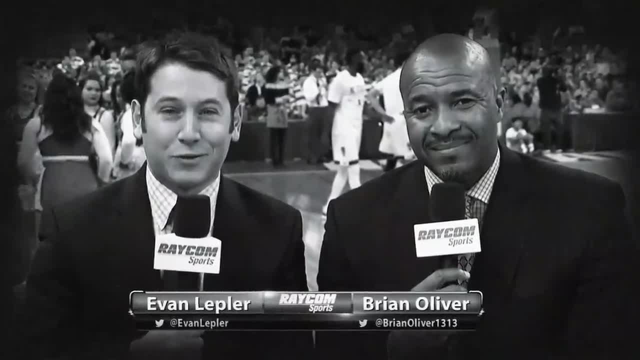 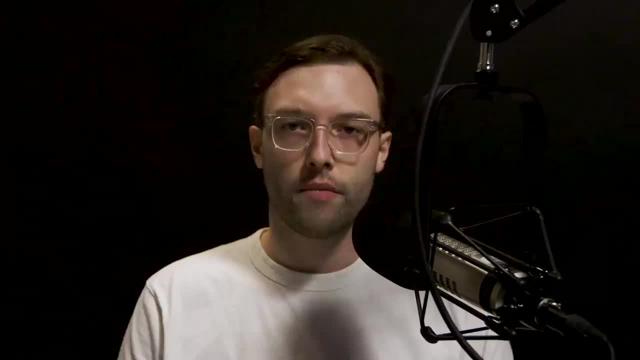 maybe they were jinxed by Evan Leppler and Brian Oliver, who tell us three minutes into the game: Evan, both of these teams are tops in the league in scoring and you're going to see a frenetic pace of going back and forth. And oh how those teams go back and forth. What exactly happens over the? 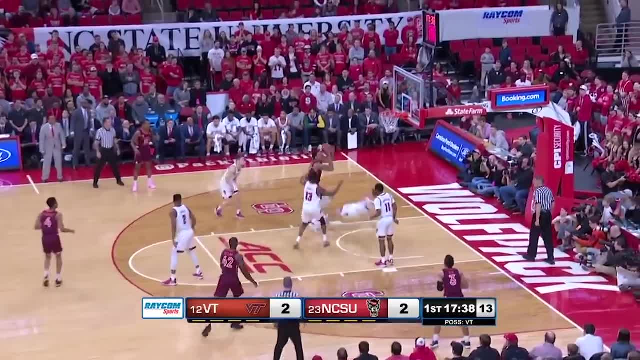 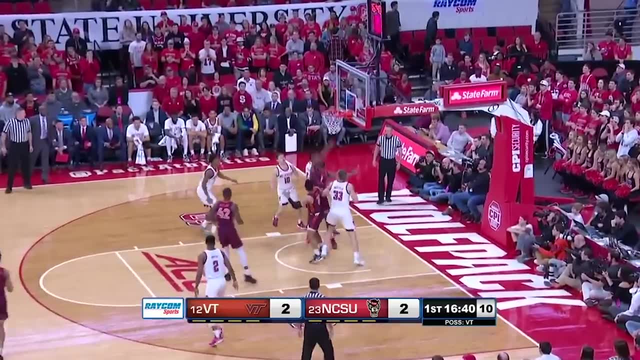 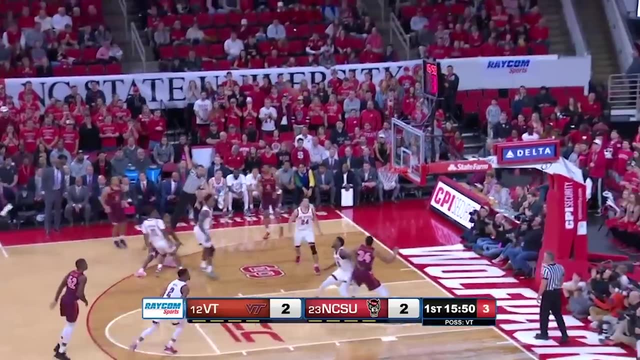 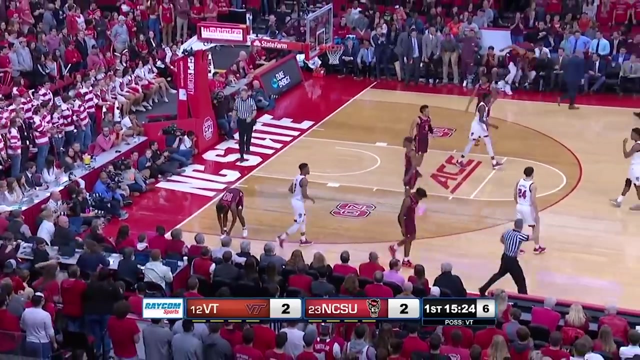 following five minutes of game time, Only this Foul and a turnover. Miss Turnover, Miss Foul, Miss, Miss Turnover on this absolutely hilarious out-of-bounds pass from Markel Johnson. Goodness gracious, Someone was open, but he was in the third row. 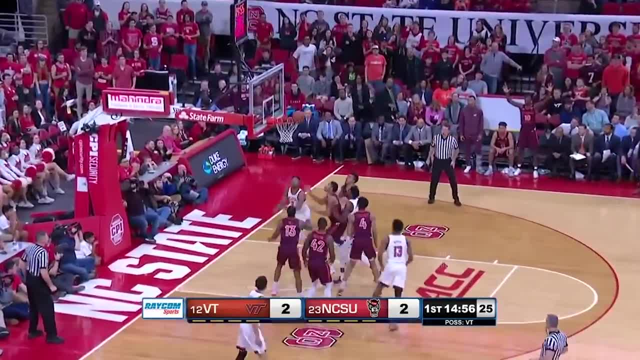 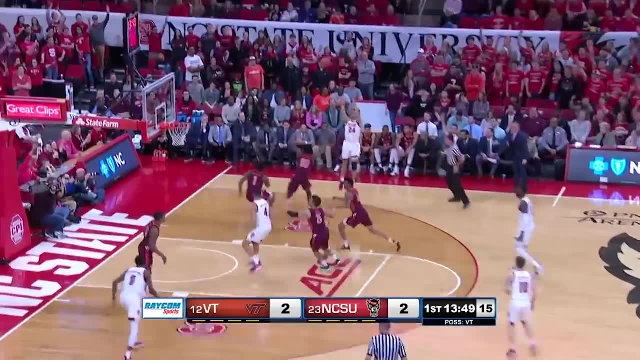 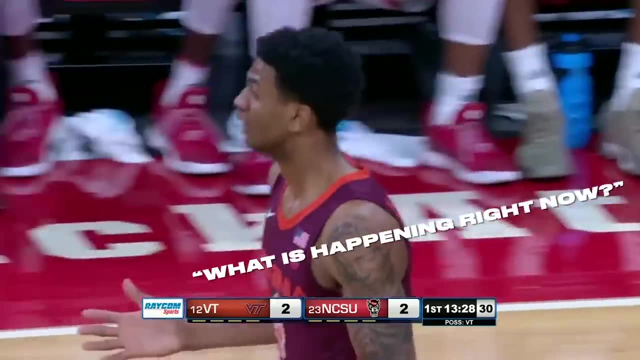 Turnover, Miss, Miss. Offensive rebound Foul on NC State. Turnover, Miss, Turnover. And that, by the way, is Tech's seventh turnover of the game so far. There is, if nothing else, some defense Now before we finally get to the next points of this game. 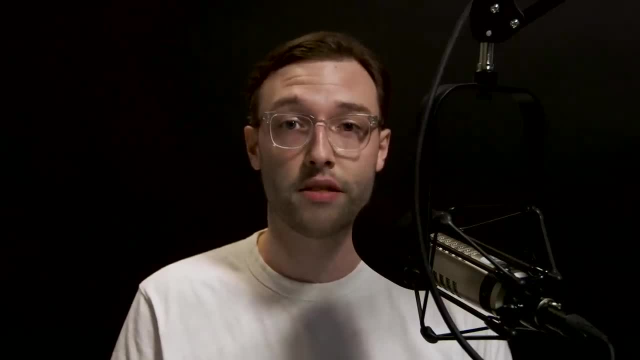 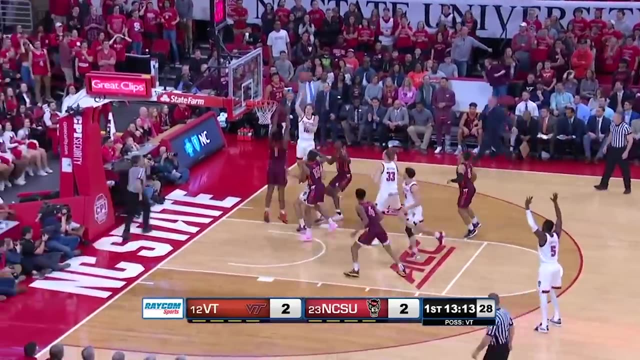 I want you to take a look at NC State's last possession before that happens. We've got a missed three-point jumper by Braxton Beverly Wyatt Walker with the offensive rebound back to Beverly for a missed jumper, then a missed tip and a missed put-back attempt by Walker. 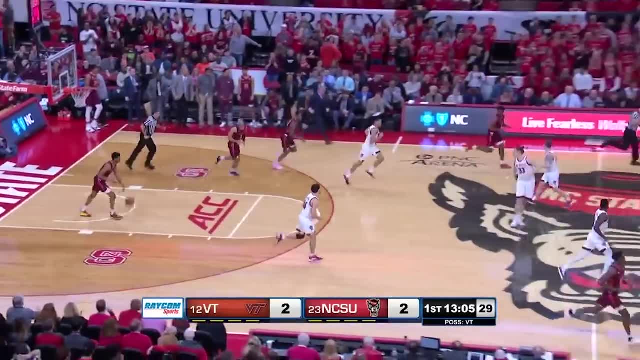 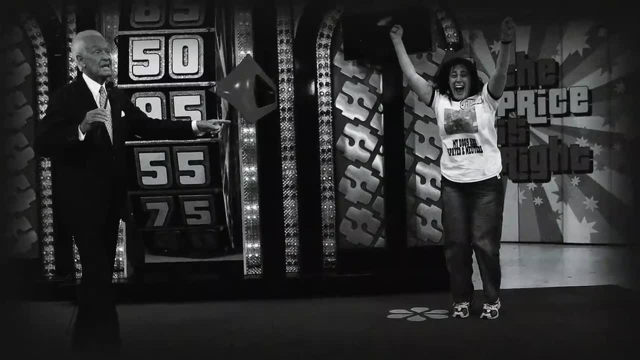 Four chances. None of them confirmed That sound you hear from the crowd. after all of this is the same exact sound you hear from an audience dealing with a frustrating contestant on the Price is Right. Joy, Joy, Help her audience. She needs help. 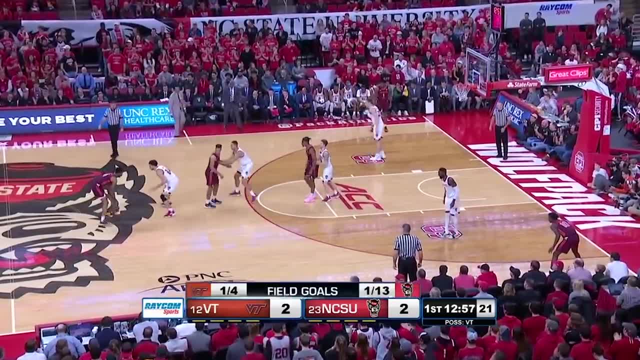 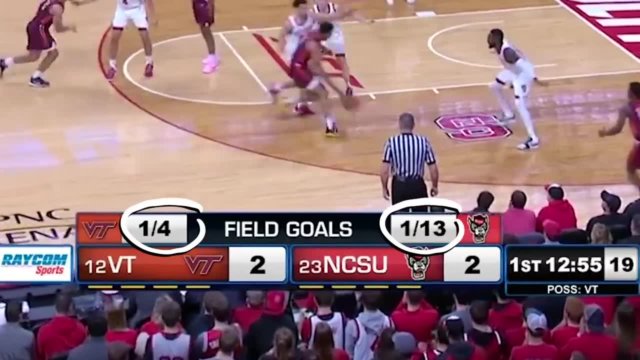 We're almost at the much-hyped debut of a second made shot by either of these teams. but first I just want to quickly point out the stat line graphic that the broadcast puts up right before it happens. That is crazy Here. finally, with 12.54 left in the half. 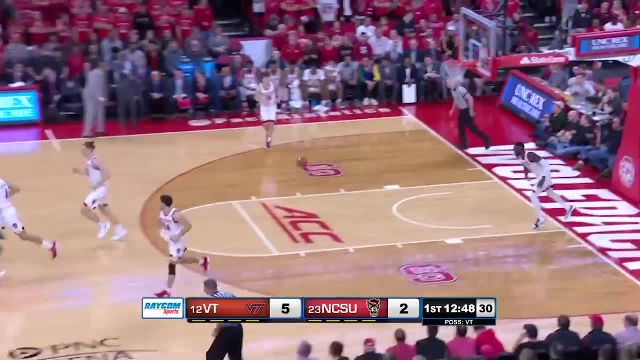 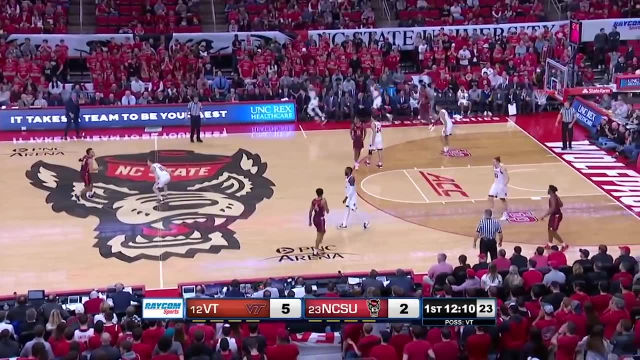 the Hokies' Isaiah Wilkins nails a three-pointer and the home crowd cheers simply because they finally saw a basketball thing happen. At this point, the analysts would like to remind you again that these are Two of the better field goal shooting teams, ranked first and third in the conference. 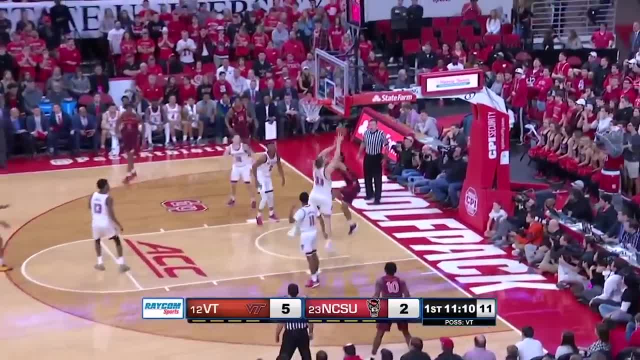 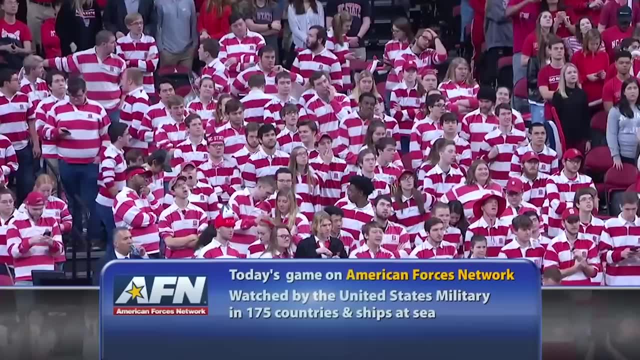 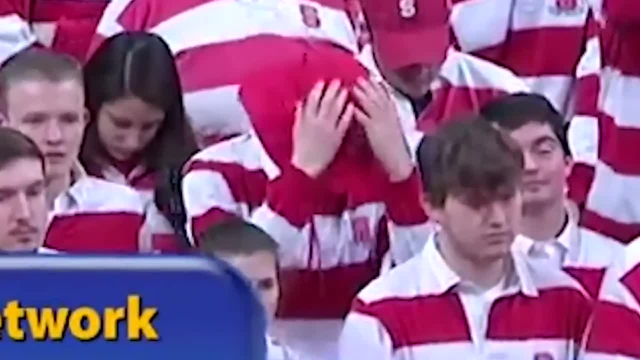 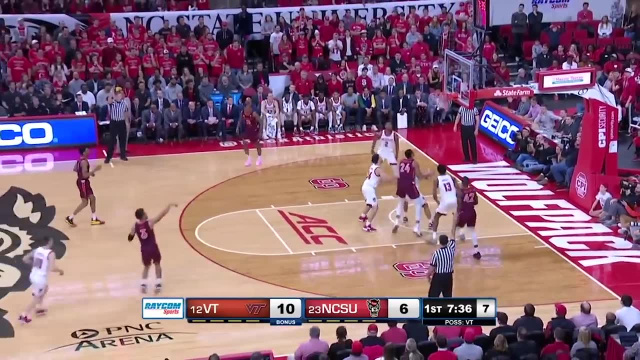 so you can pick out your favorite. This one's mine, because I know how much it sucks to wear your best hat out on the town for nothing. Later, with 7.30 left in the half, a Hokies' three-point jumper brings the game to 13-6,. 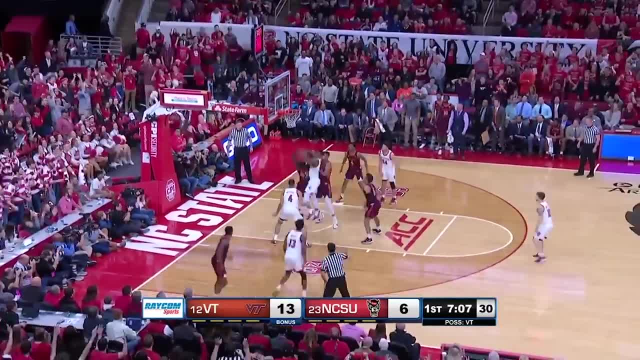 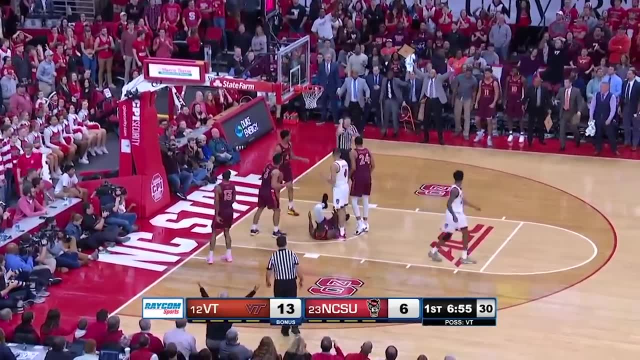 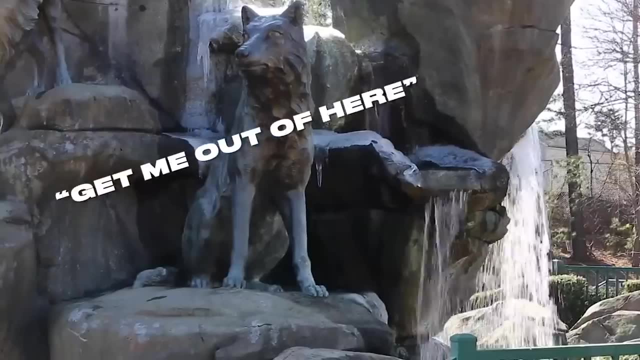 and the Wolfpack respond with another brutal possession consisting of five shots and five misses. A few more feeble attempts at scoring are punctuated by some actual buckets, but eventually both teams limp into halftime with a combined 34 points for a score of 20-14, the fewest combined. 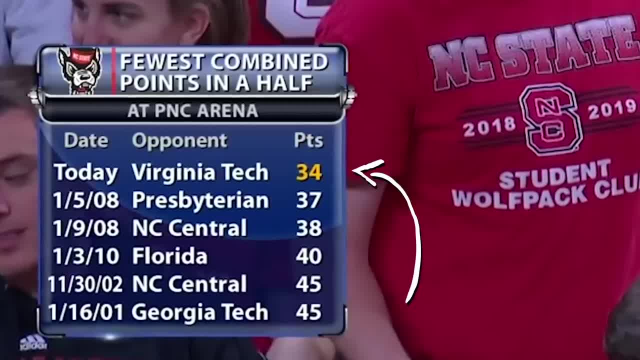 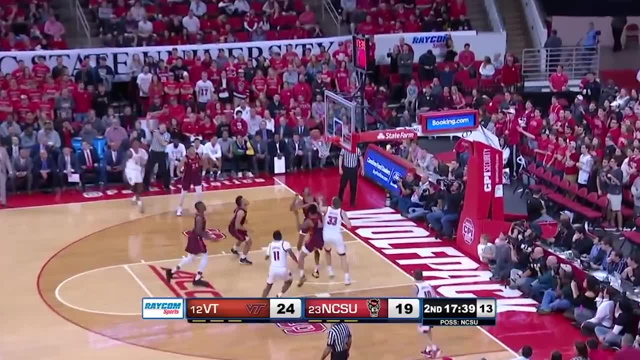 points in a half that PNC Arena has ever seen. But yes, despite NC State's abysmal shooting performance, they've managed to keep it within six. On to the second half, where NC State quickly treats us to yet another impotent possession, with multiple shots that result in nothing. 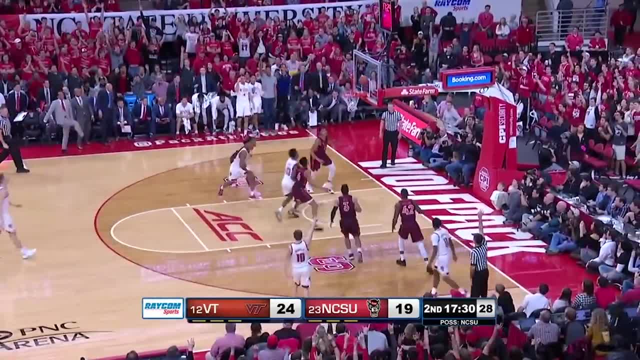 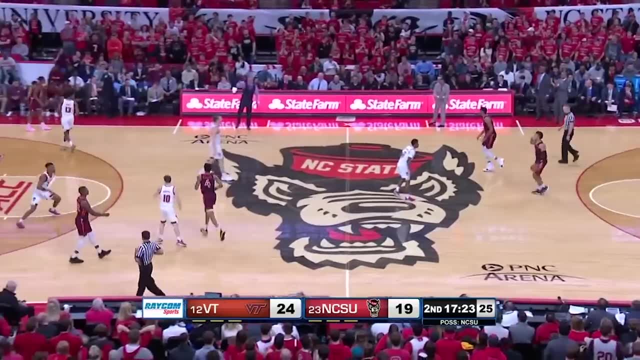 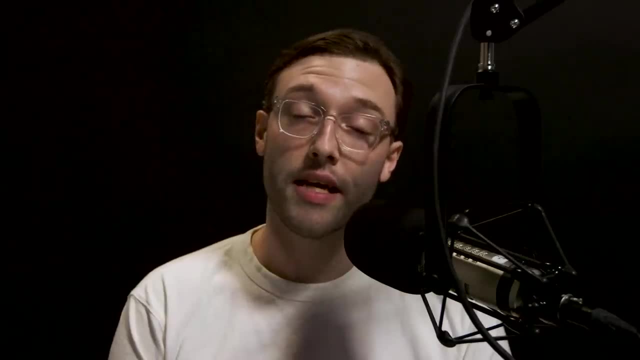 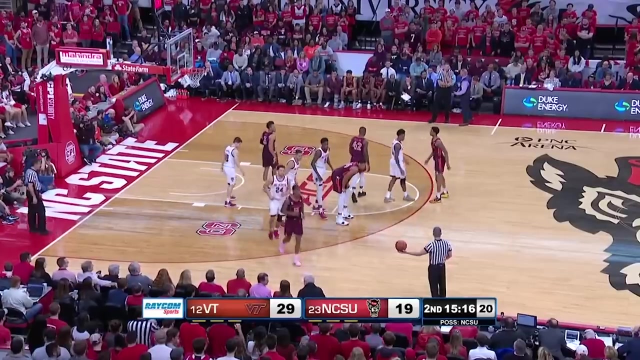 including yet another miss from Braxton Beverly, who is scoreless so far today. Sooner or later, we're going to realize that that assumption is incorrect. At one point the broadcast, in a moment of relative quiet, picks up a frustrated fan who acutely expresses what we're all thinking. 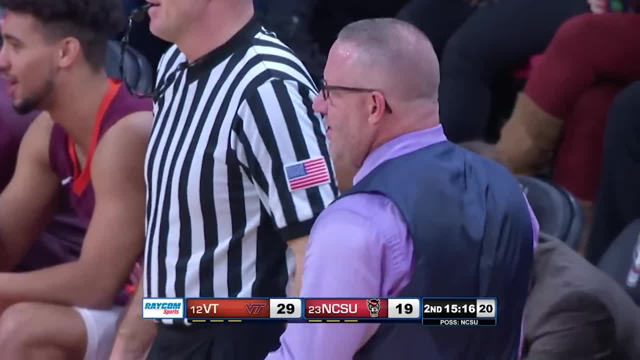 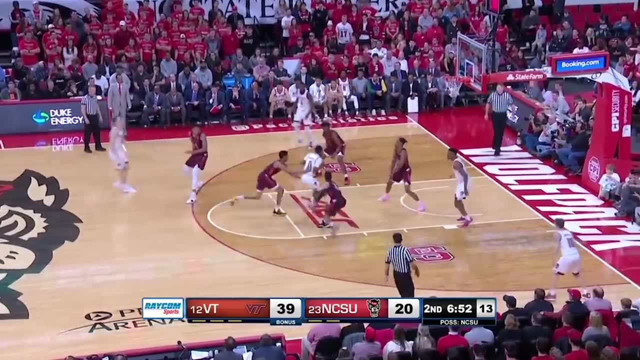 Friend, this is not basketball, This is something darker, more sinister. That brings us to 6.50 left in the half, And I want you to really take in this Torin Dorn layup, as it will be NC State's last field goal. 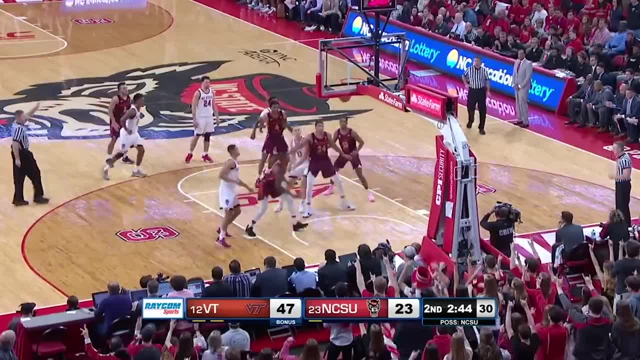 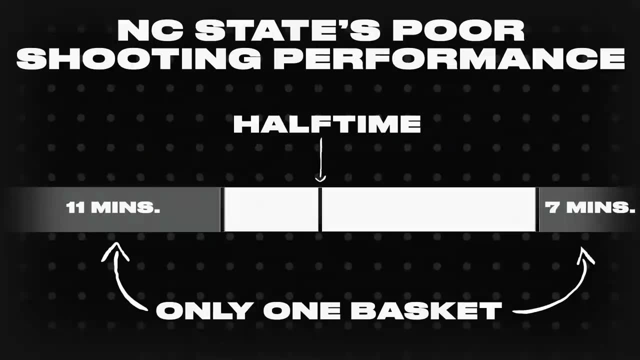 of the game. They'll score two more points on free throws before the game is up, but I think it's kind of neat that they managed to bookend this game 11 minutes at the beginning and 7 at the end, for a total of 18 minutes, with only a single made shot, And that's kind of it. 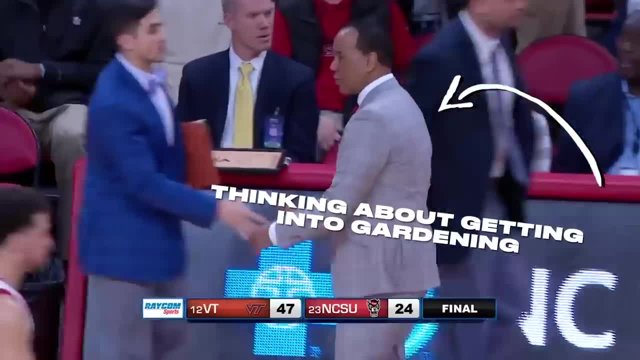 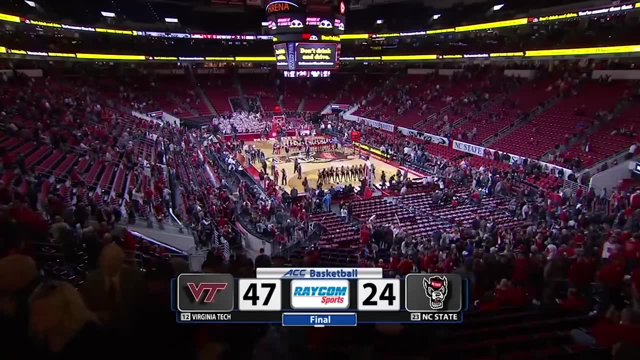 The analysts wonder aloud: Could this be the lowest scoring game in Wolfpack history? It's close. The band gallantly sticks around to play one final derd to a mostly empty arena and this game, such as it is, is over. 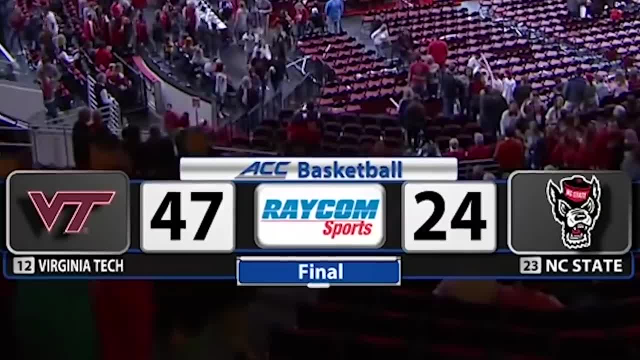 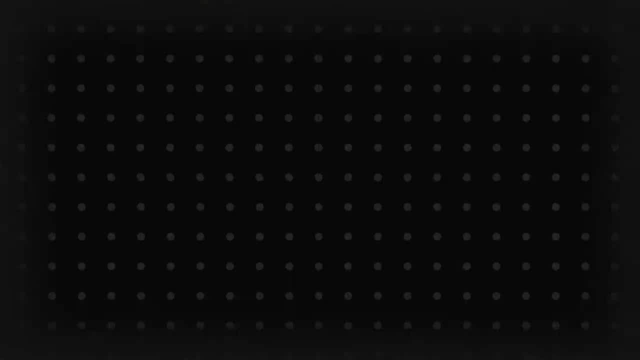 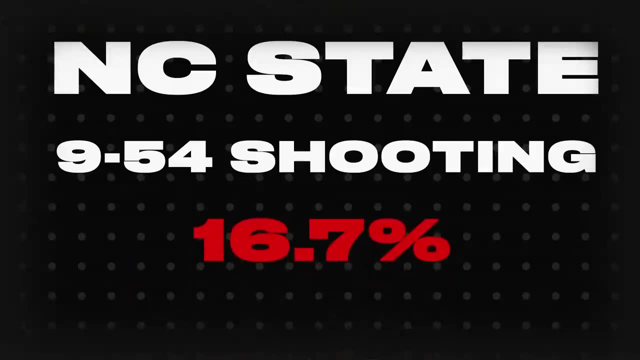 The final score: 47 to 24.. 47 to 24.. Yes, that is a real basketball score. Here are a few things that are true. The Wolfpack went 9 for 54 in this game, a shooting percentage of 16.7.. That is the lowest percentage in the history of the ACC. 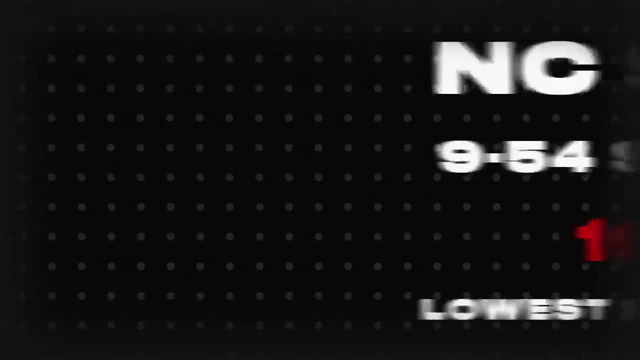 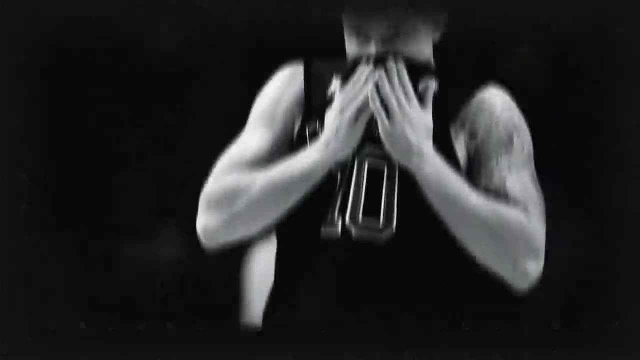 which was formed in 1953. You'd think they would make some adjustments at halftime, but in fact the Wolfpack shot 194 in the first half and then dropped to 130 after halftime. Braxton Beverly went 0 for 12 from the field and 0 for 9 from behind the arc. a big fat goose egg of a game for him. 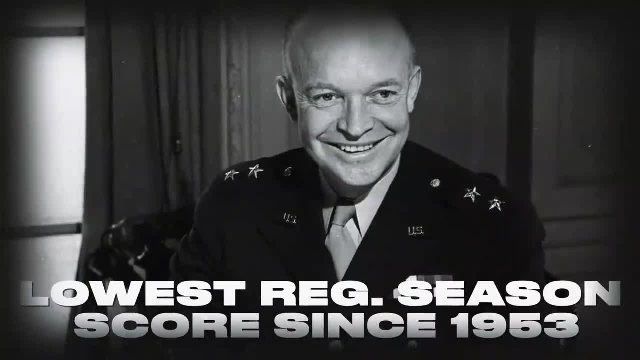 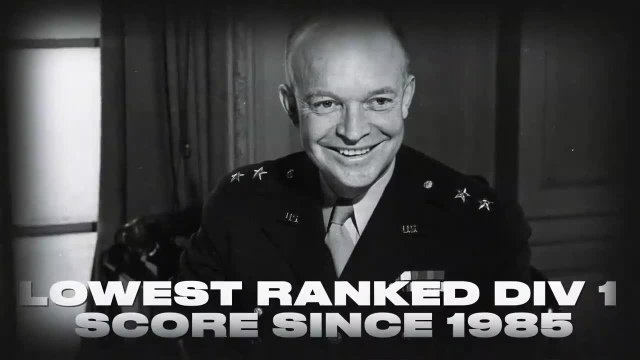 It's the lowest scoring game NC State has had in a regular season game since Dwight D Eisenhower was president, And it's the lowest scoring game of any ranked Division I school since the shot clock was established in 1985.. But a question remains: Is this truly the worst college basketball? 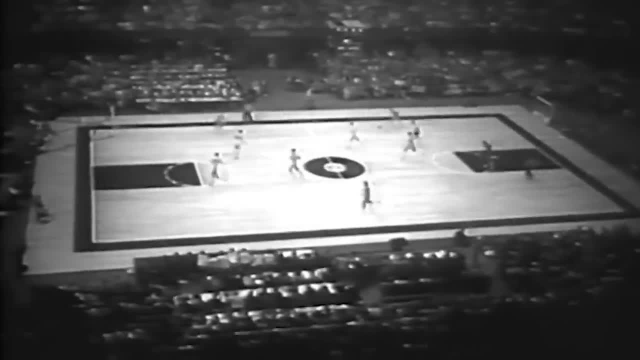 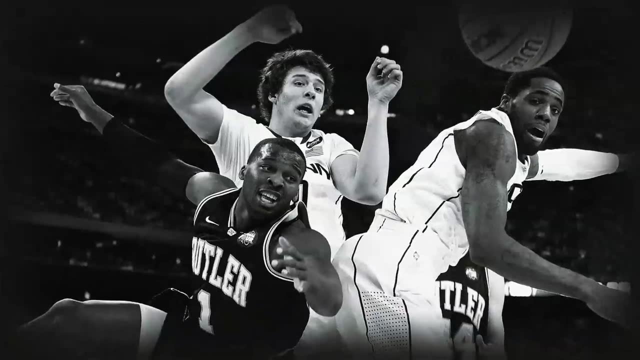 game of all time. There are thousands of NCAA games that get played every year, and basketball has been played at colleges for the better part of a century. Surely there are other contenders. Take, for instance, the 2011 NCAA championship between Butler and UConn, which ended with the fewest combined points. 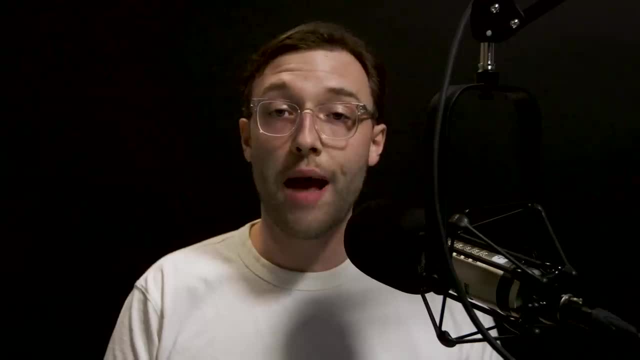 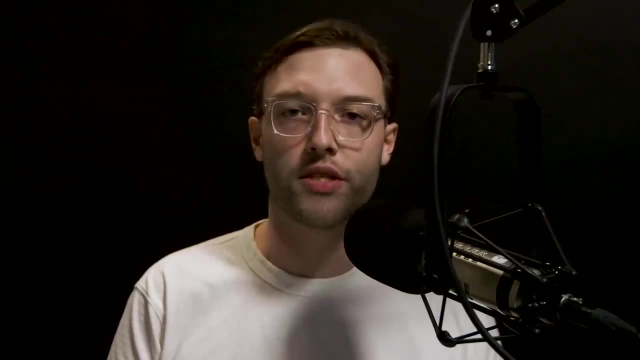 in a championship game since 1949. Or perhaps a 2013 game between Northern Illinois and Eastern Michigan, which, well, you know what? I'll let eyewitness John Boyce tell you about that one, John, 2013, Northern Illinois versus Eastern Michigan. There are. 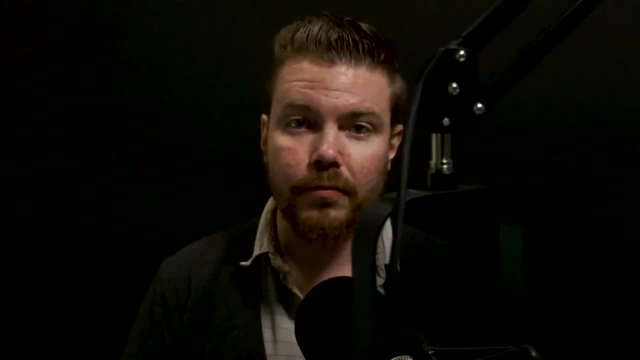 three things I want to tell you about this game. The first is that Northern Illinois scored four points in the entire first half. The second is they went one for 33 from the three-point range and only hit their one with two minutes left in the game. The third, my personal favorite. 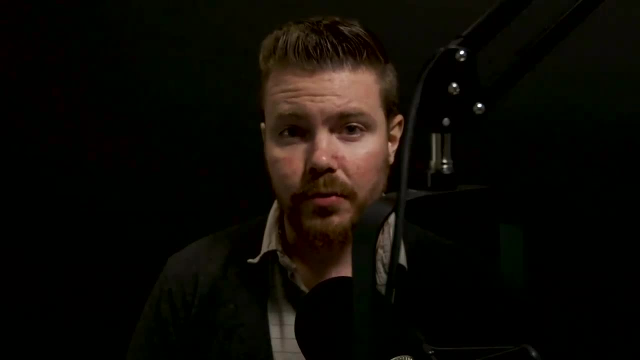 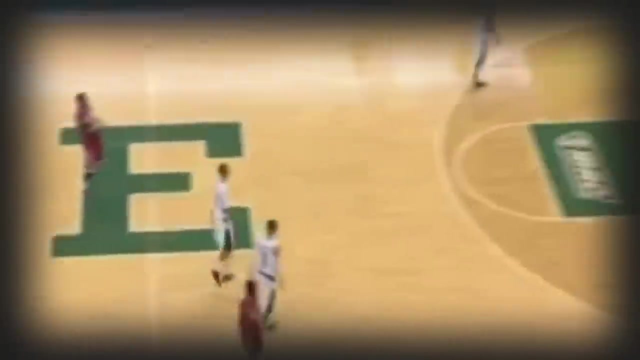 one of those threes was an air ball. A Northern Illinois player was supposed to rebound it. He was under the net. He watches it come down. Instead of putting his hands up, he puts them down. slack at his sides. He watches the ball hit him in the chest and bounce out of bounds. 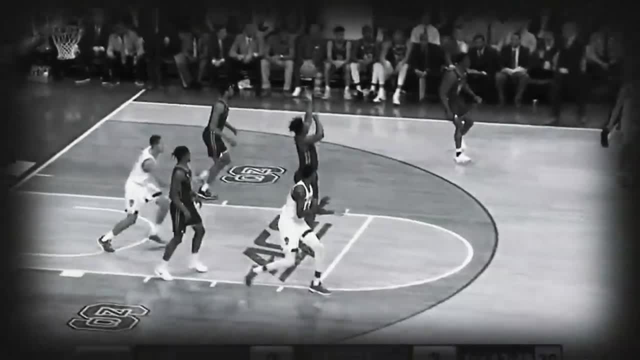 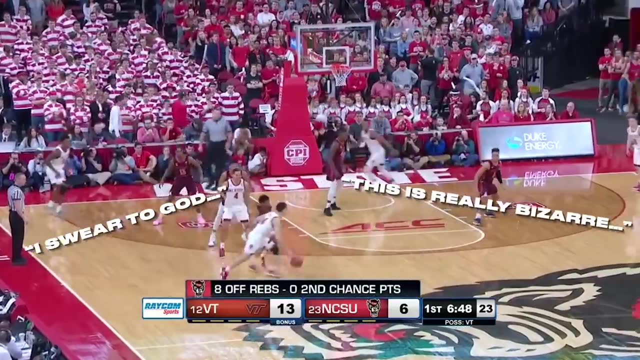 Greatest game ever. Total stinkers, to be sure. Something to be said for a game in which the play-by-play guys turn on these kids early and often. I swear to God, this is really bizarre. Two teams that can really score. Believe us. 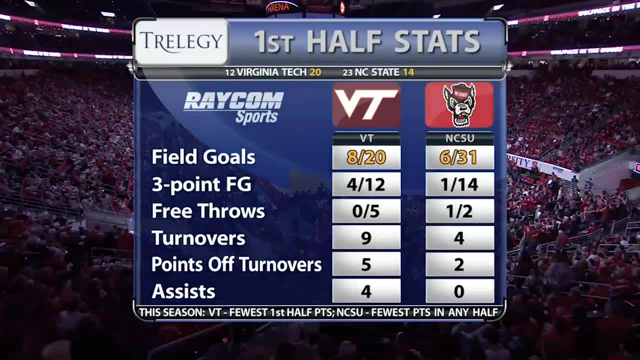 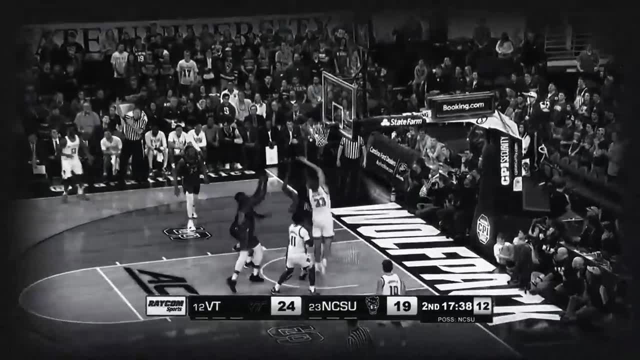 please, We'd understand if you'd like to avert your eyes. Indeed, But like any good train wreck, sometimes it can just be impossible to tear yourself away. So the next time you fail miserably at the most basic task expected of you. 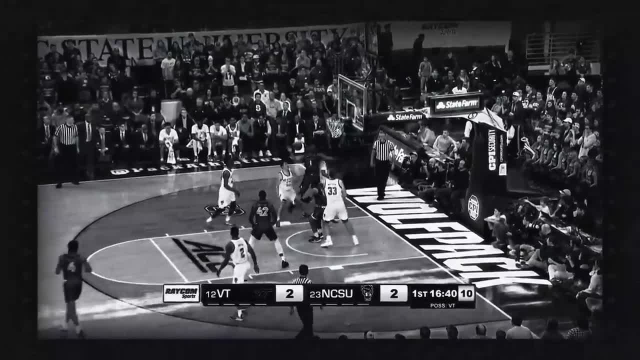 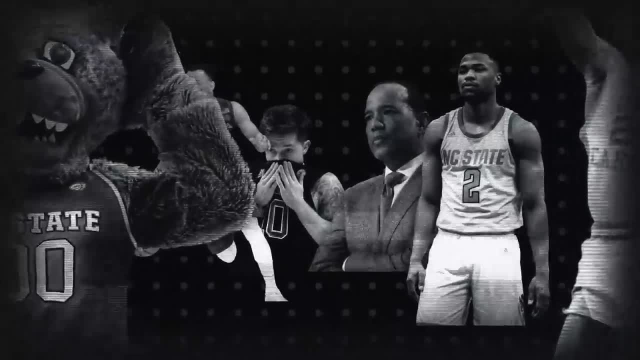 just remember that one time, and not very long ago, an entire college basketball program was incapable of accomplishing even the most basic task possible, Even the most basic element of the game: Putting the ball in the basket. And you know what? Life goes on. 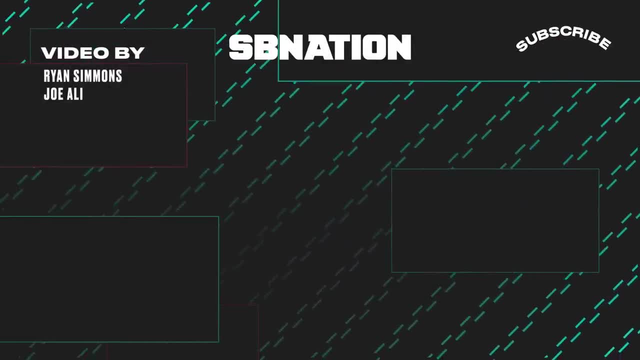 Thanks for watching. Don't forget to subscribe to SB Nation, And if you want to see more about that awful 2011 UConn Butler Championship game, we've got it for you here, Or you can check out another one of our SB Nation videos.